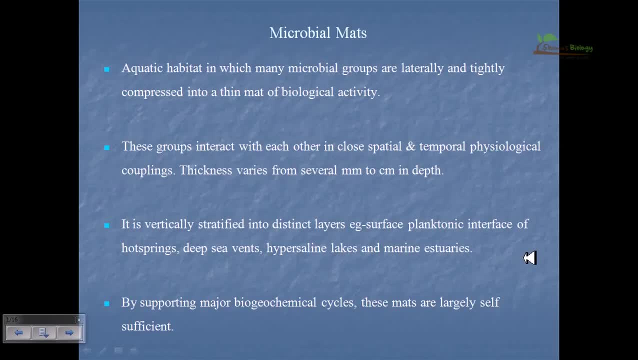 Welcome back, friends. In this video we will be talking about, more importantly, about the microbial mats and the biofilms, and these biofilms and the microbial mat, which are the organization of bacterial communities and different microbial communities, and what are the importance of making these microbial mats and what we can derive from the presence of. 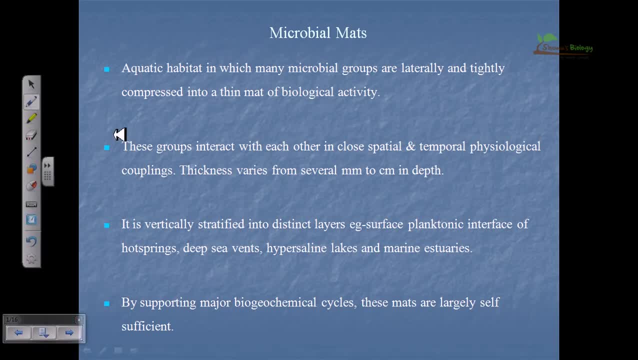 these microbial mats and all those presence of those community structures called biofilms. Now, actually, microbial mats are aquatic habitat for microorganisms in which many microbial groups are laterally and tightly compressed into a thin mat of biological activity. So we can see the mat in this way that we are having a rock suppose example. and on to the top of this rock. let me 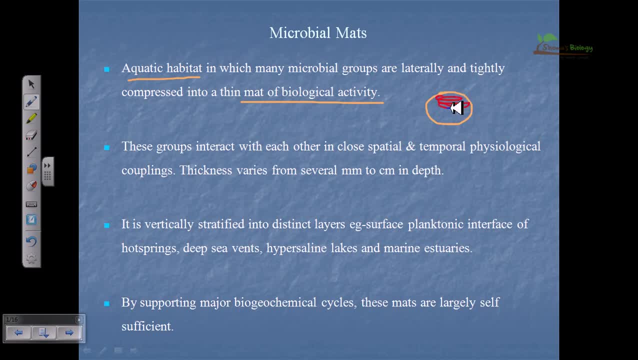 change the color. okay, on to the top of the rock. we are having a rock, suppose example. and on to the top of this rock: we are having a rock, suppose example. and on to the top of this rock: we are having a rock, suppose example. and on to the top of this rock: we are having a rock. suppose they are different. 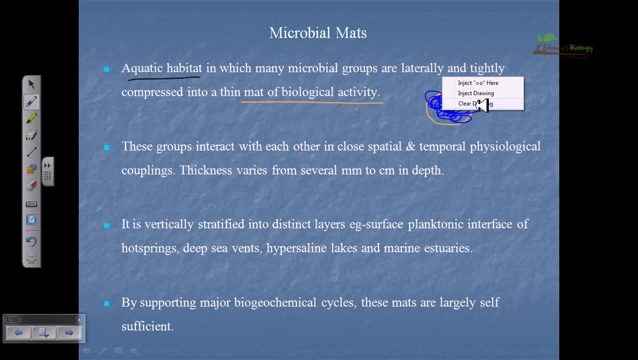 different microbes are placed together in this way is to take it okay. so they placed in different ways like that, and what they're doing, they're interacting with themselves. so we can say this: this mass are in a whole tiny ecosystem for those microorganisms and we can find different. 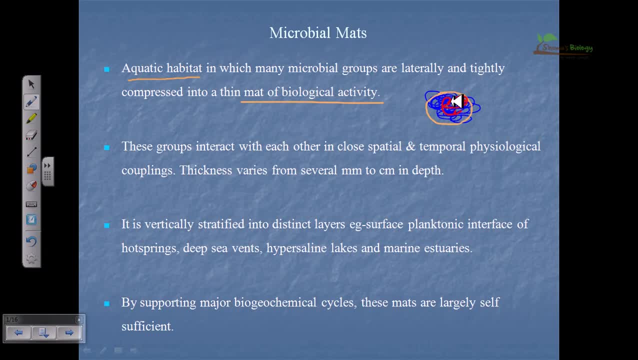 biological activities are going on, going on on this match and they're having interactions. now these groups interact with each other in close spatial and temporal physiological coupling stages. okay, now the thickness of this match normally varies. it varies from several millimeter to centimeter can vary. so you can see the small bacteria, small microbes, are very, very 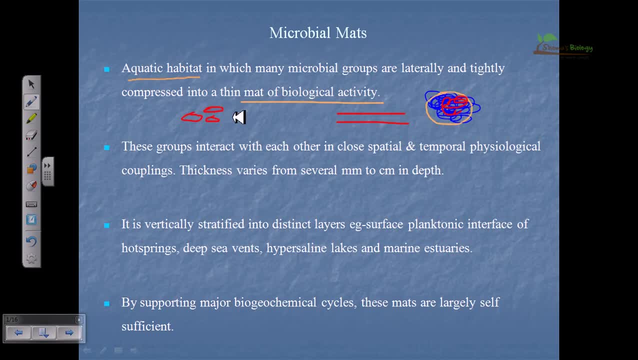 thin, so thin that we cannot see them without rare eyes. but when they interact with themselves and couple with themselves, they will form like this: one centimeter or two centimeter or three centimeter or couple of millimeter depth containing mats. so there will be huge amount of bacteria present in. 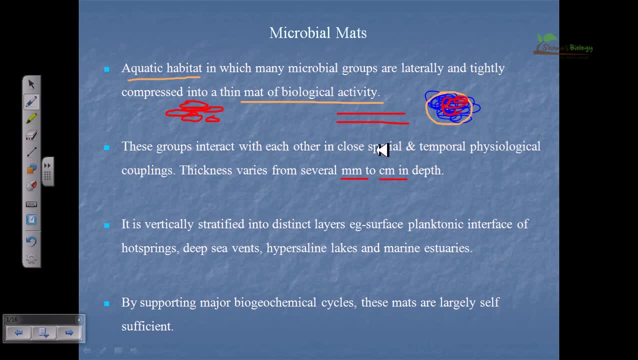 this match. okay, now what happens in this case? this mat are producing different layers among the sea rocks in different orientations, like, for example, the surface planktonic interface we can find in case of hot spring. you can have in the hot spring. bacteria cannot live on to the deep water because 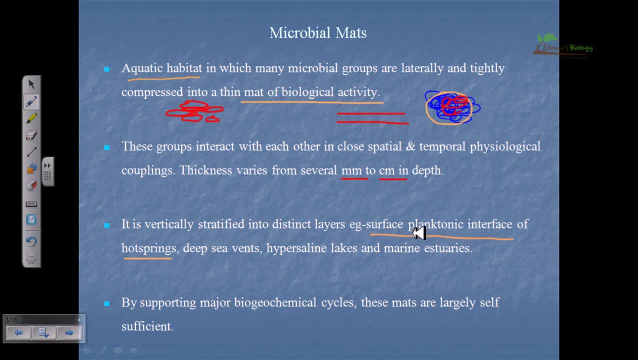 that was really hot. so they have to live on to the surface. so they have to live on to the surface. so maybe they don't live over or they may live at Wisconsin or vedere with the earlier sources, but they are version of the surface. so this circle, so that may even end up be the surface of 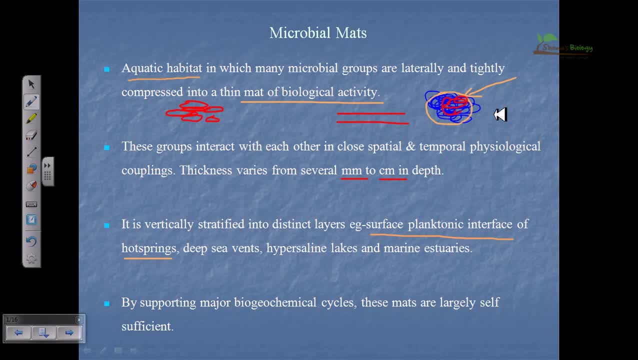 this hot spring or surface layer of this hot spring, and there we can find this microbial mats. now, this microbial mats are actually helping them to resist the environmental stress. there's another very, very important part, just like the biofilm, so the activity of microbial mat and the 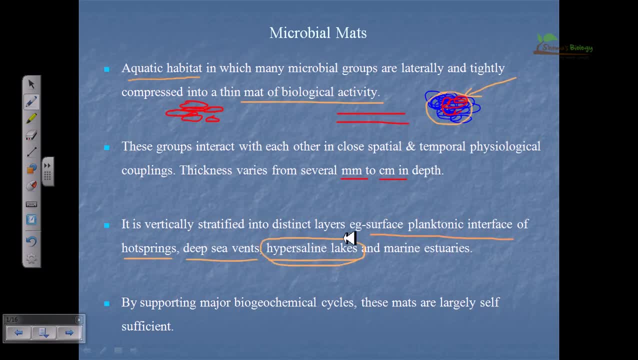 biofilm remains more or less the same. okay, now also, you can find this microbial mats in the deep of sodium chloride and in case of the deep sea vents, in case of deep sea vents, we are having higher pressure, very, very higher pressure is going on, and in hot hydrothermal veins or hot springs, we 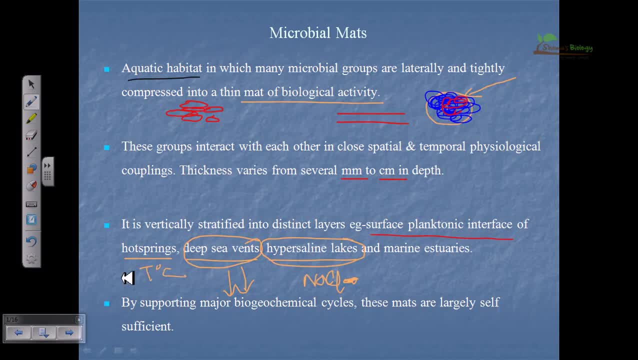 can have very, very high temperature, so temperature is very high in those cases. in all these cases we can find the harsh environmental situations and microbial mass are found there because normal type or bacteria cannot live on their own in this type of dangerous situations, so they need to live with. 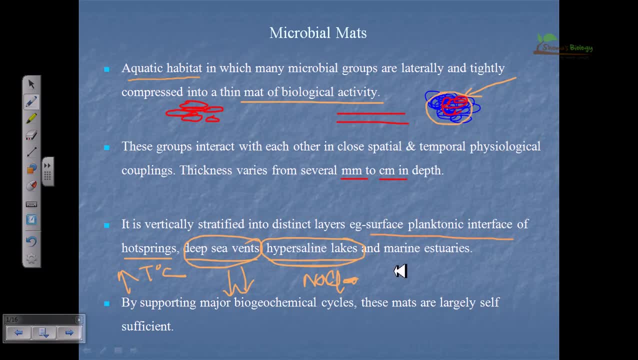 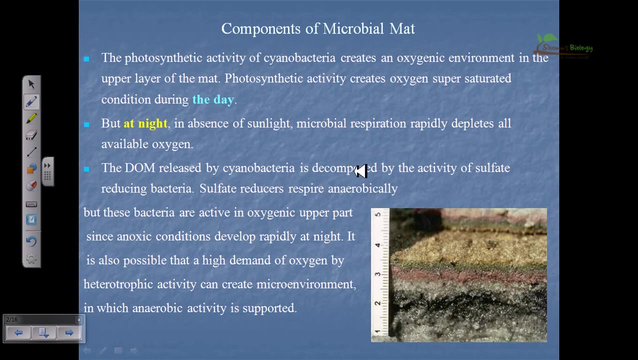 themselves. they need to live by forming communities together or adhering with their own cells, and that's how we can find these different types of microbial mats. okay, now let's move on to the next slide. now, here we can find the components of microbial mat that you can find here: the 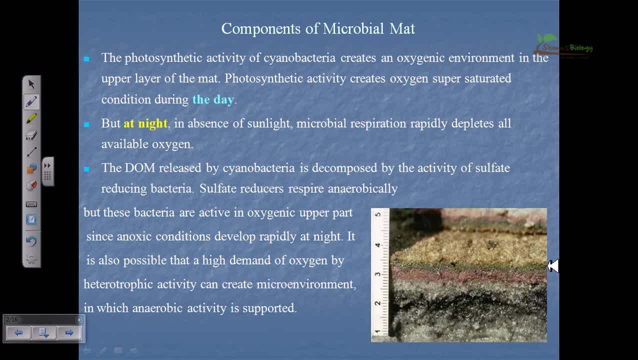 photosynthetic activity can be shown in this microbial mass. you can, if you look at this microbial man. this is the top layer where you can find slightly greenish type of layer, and this greenish layer suggests us that these are the microorganisms which are having the chlorophyll molecule because, because they are having this. 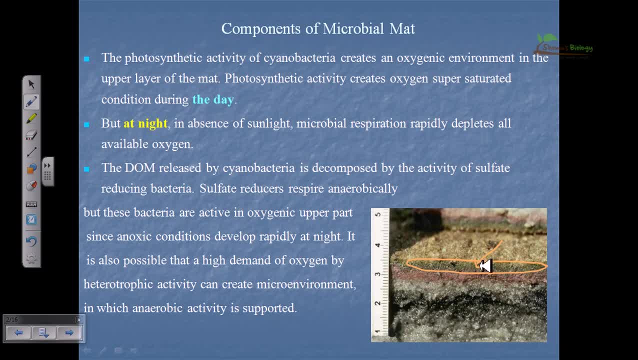 chlorophyll and they are getting the sunlight, as you can see in this picture. they can easily go through the photosynthesis. okay, so the photosynthetic activity can be go, can be carried out by this surface layers, like those bacteria, like cyanobacteria. they can create an oxygenic 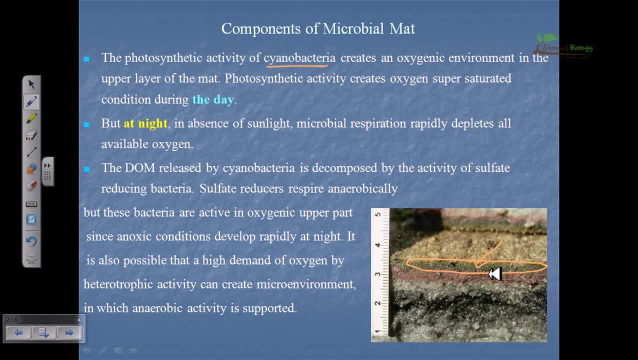 environment, in this microbial mass, and they can be carried out by these surface layers, like those bacteria, like cyanobacteria. they can create an oxygenic environment in the upper layer of the mat. okay. and photosynthesis, can we go? okay, can be taken through the daytime, right, but at night, in the absence of sunlight, microbial respiration rapidly grow, goes on and 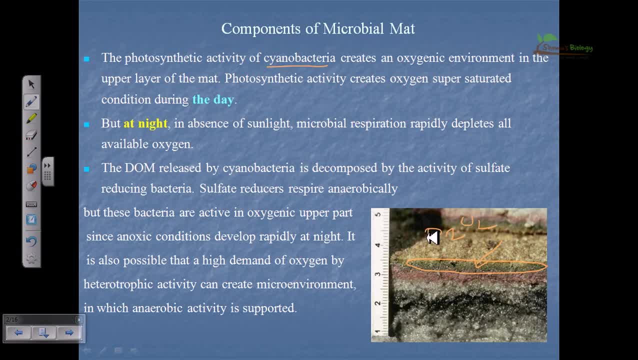 as a result of this respiration, all the oxygen that are being produced during the daytime via the photosynthesis are depleting. so they, they, they start to take out, take out all this oxygen. so the lower layers, which are which cannot do the photosynthesis, and the other layers of bacteria. 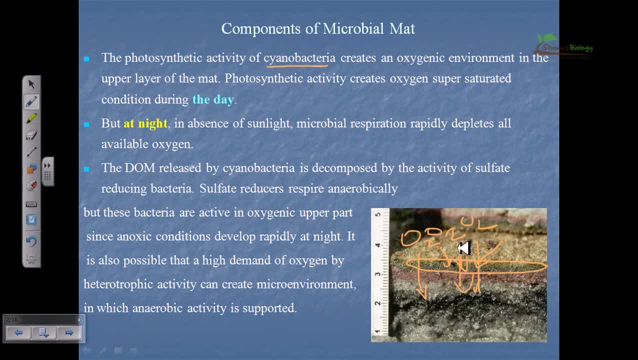 have to take this oxygen because they need to go carry out their respiratory cycles, so for that, they will take up this oxygen and, as a result, oxygen depletion will take place at the night time. okay, so this is another very important thing. so by by looking at this structure of a bio, 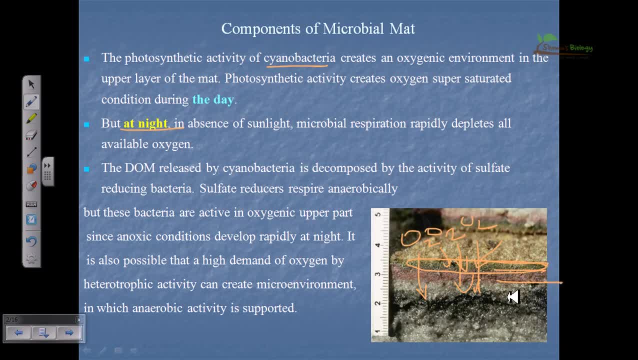 of this microbial mat, you can find different layers, and among different layers we can find different types of bacteria. and another very important thing is that you can find different types of colors. in the top layer we are having the green color, such as the presence of chlorophyll. 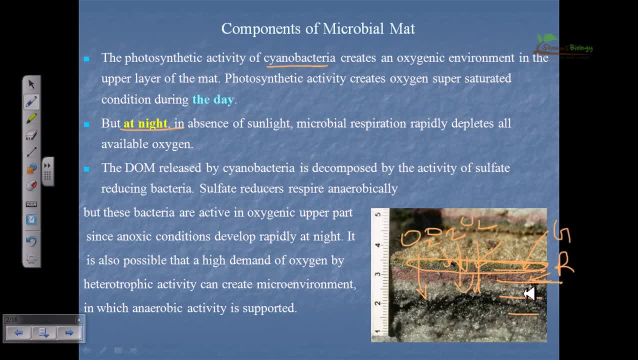 bottom layer. we are looking at the red color and this layer is the black in color, so they are different. so carbon compound is very, very higher amount in this black layer. red color suggested that it may contain carotenes or carotenoids and all these things they can. 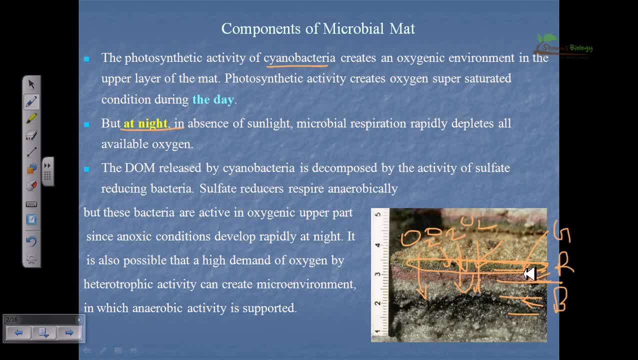 also help them to go through the photosynthesis. in this case, sometimes these are the antenna pigments, as we know. okay, so the presence of different pigments also tell, also tell us about how this microbes are interacting with each other and how they are living, how they can gather energy for. 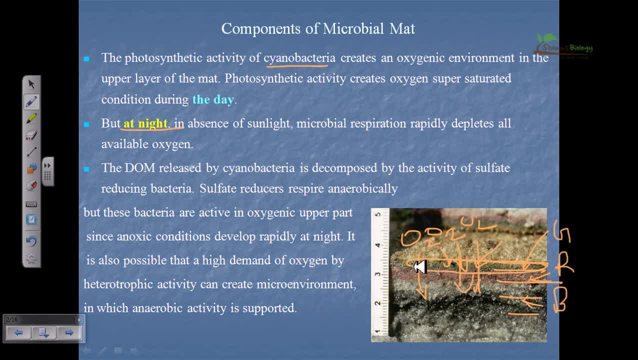 their living. okay, so these are very, very important about. okay. now, what happens? the? the dissolved oxygen matter, whatever present, is there. it is released by the cyanobacteria, is decomposed by the activity of the sulfate reducing bacteria- sulfate reducing bacteria also present there- or sulfide oxidizing bacteria- whatever you can say. now, the sulfur reducers respire anaerobically, but 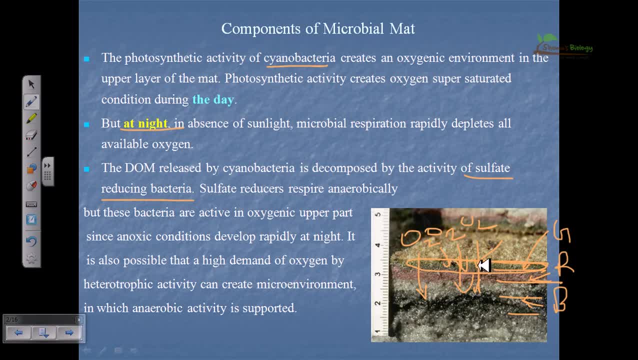 the bacteria are in active in oxygen upper part, since anoxic conditions develop rapidly at night. now it is also possible that the high demand of oxygen by the heterotropic activity can create micro environment. okay, and this micro environment are supporting the growth of your type of micro? 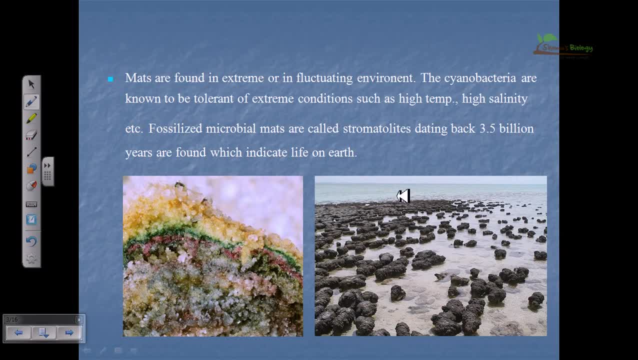 organisms. now these are the examples of beautiful microbial mats and this is a beautiful picture of microbial mat. you can find the same type of picture here also, and here also right. so you can see here the green color, what a beautiful color it is. it's a very, very much green. then the red and black and 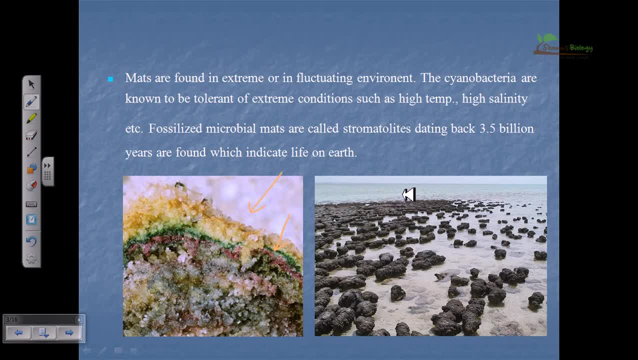 yellow and all the colorations are going on in this case- and the right picture. we're looking at the microbial net, fossils or fossilized microbial mats. now what happens? the cyanobacteria are known to be the tolerant to extreme conditions such as the high temperature or high salinity or high 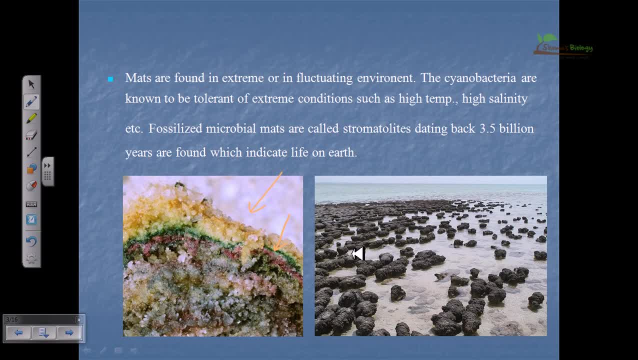 pressure. so we can find this cyanobacteria in the deep oceanic veins or in hydrothermal veins and salinity lakes. now this cyanobacteria came very, very earlier during the course of bacterial evolution. so in those situations in that those past time, the environment is not that much suitable. 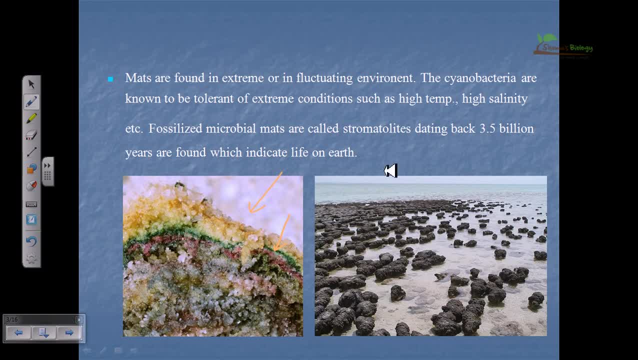 for life's growth, so cyanobacteria have to live on, uh for and and against those environmental conditions, so they adopt the situation. okay, so we can see nowadays, uh the presence of this microbial mats which are in the fossilized form, so we can find more and more cyanobacteria that 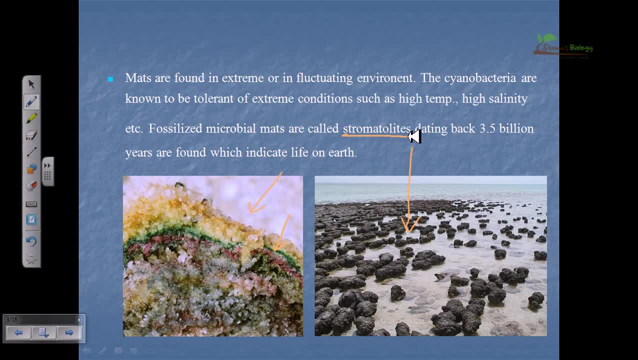 are present here. okay, and we can also call this stromatolites. it's a very, very important terminology. we can call it stromatolites, okay, the millions of stromatolites can be found here, like this surface area of this ocean. okay, now, if we date this, uh, with the help of radiocarbon dating or some other, 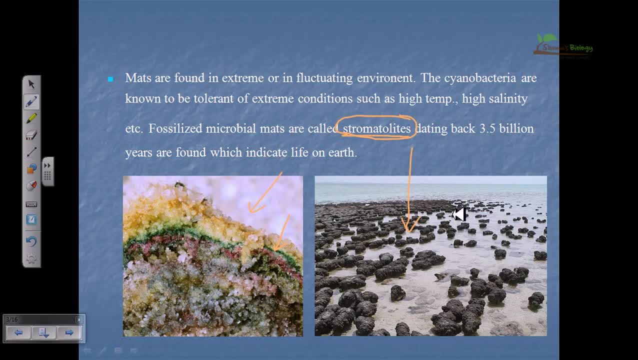 type of carbon dating techniques, we can find that, uh, the age of these stromatolites are more, more or less, 3.5 billion years. okay, so that again suggests us the origin of life. that again suggests us the origin or the presence of the cyanobacteria almost 3.5 billion years ago. okay, so this is very, very important. 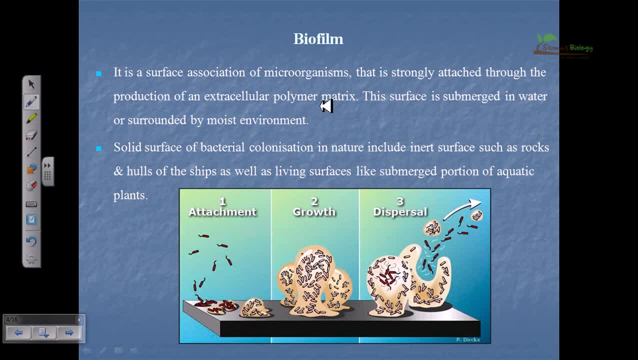 okay, now let us talk about, uh, biofilms. now we have talked about microbial mats. uh, these microbial mats are nothing but a biofilm arrangement. okay, because biofilm means we are having more and more biofilms and we are having more and more biofilms and we are having more and more. 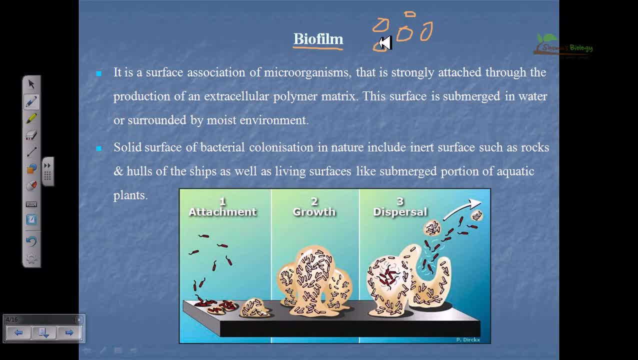 bacterial cells of same type of bacteria or sometimes different types of bacteria. they will come and interact with each other by secreting chemical components or adhesions, and these adhesions will hold them together to form matte like structure and they will form a coat outside. 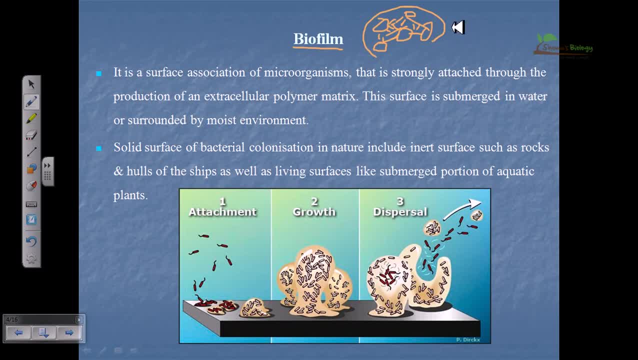 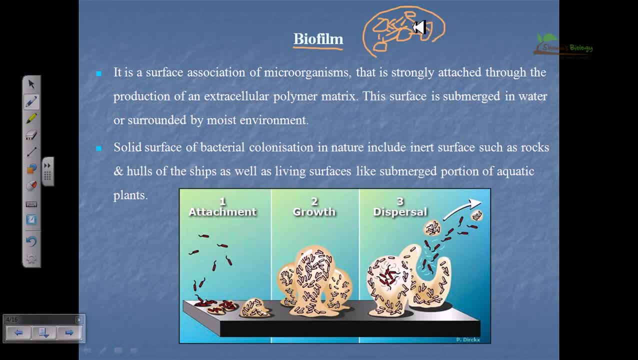 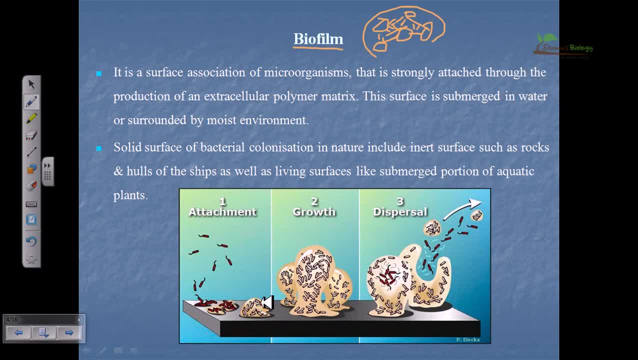 with each other. they are attached to themselves, so they are very, very strong arrangement. so this is into a suppose, a solid phase. so definitely i have missed this part that they must have this solid phase right. so they need something to grow on and this is the solid phase. so this red color thing is: 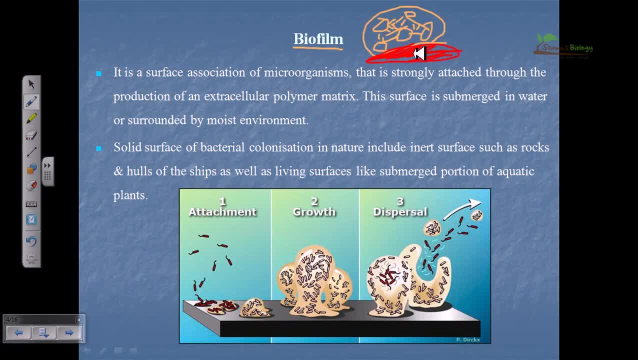 a solid phase and onto which these microbes are growing. okay, now, here in this picture we can find three different stages of biofilm. first stage is the attachment, and the attachment deals with that. all the bacterial cell will come and secrete some chemical facts which are adhesive like structures. 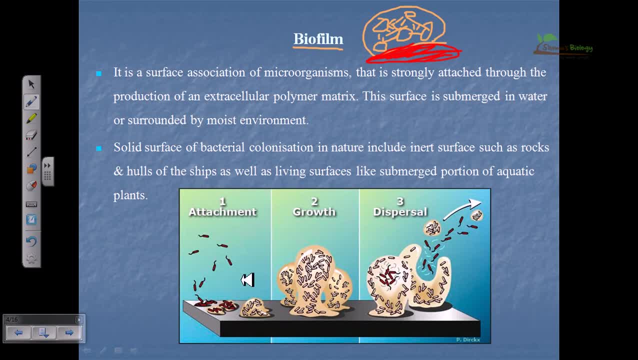 which can hold on to the hold on to the bacterial cells together, and then they start secreting all those extracellular components, like proteoglycans or polysaccharides or mucilage, like layers which are very, very slippery and very, very adhesive. so they start to make a covering of all those. 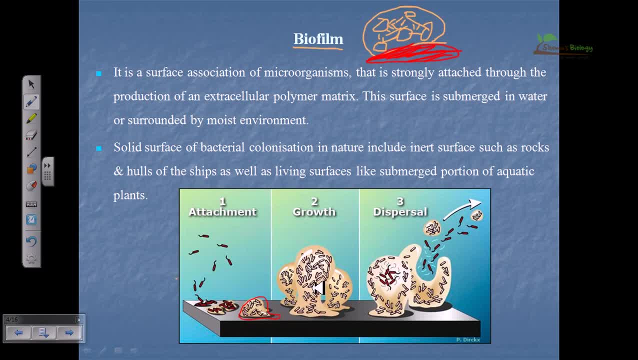 bacterial cell and they'll make a cover, in this case, okay, and this cover, uh, then finally go, or then bacteria cell will start to divide in between this cover and they start secreting all those machineries. and the structure of this mat is growing on and on and on all the time you. 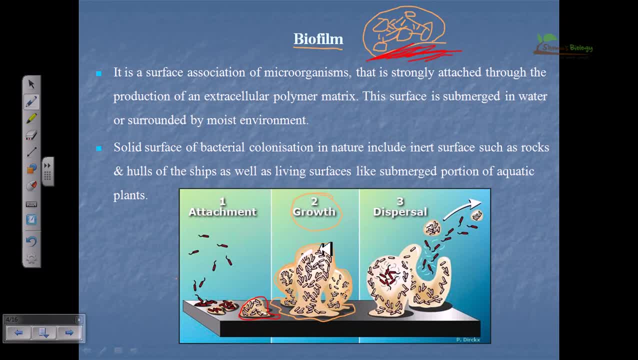 can see here it is growing. so the second phase is the growth, and after the growth it must be transferred to some different place because it it definitely need to be circulated from one place to another place. it need to be moved because all the other bacteria are freezed in this particular area. 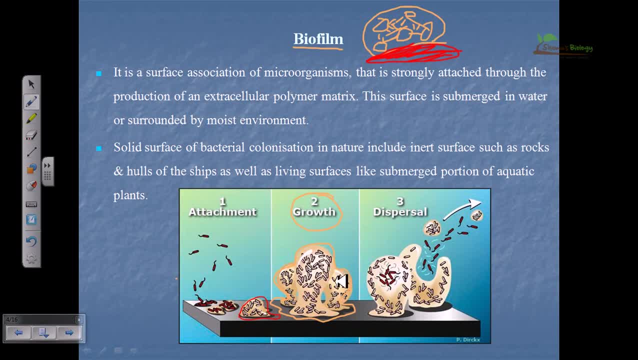 they can move on between themselves, but in this area they are totally free. so then they must be carried into some other place. so the third stage is a dispersal. in this dispersal stages, this, this uh glycocalyx layer, or or uh, this, this polysaccharide layer is 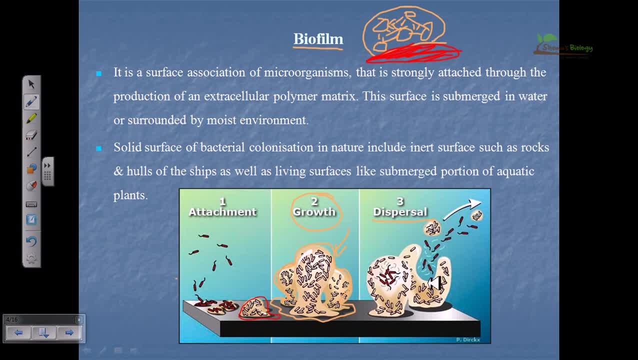 bust and cleaved and small uh vesicle can carry million of bacteria from one place to another place. okay, so the third stage is a dispersal for that. okay, so they are growing in, in uh in an amount, then they are dispersing themselves and then in, then this: 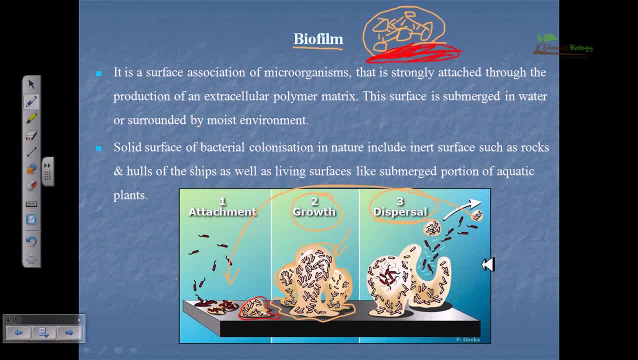 these things will go on and again attach to some other place and the whole cycle will go on. okay, so this is the thing, but the most important thing is that they must have the solid surface or the surface for their attachment, because they will be stationary. second thing is that the 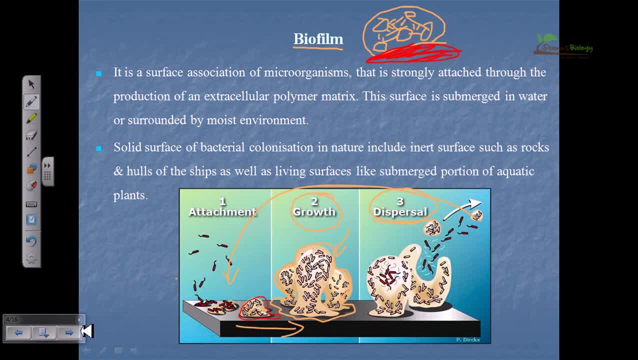 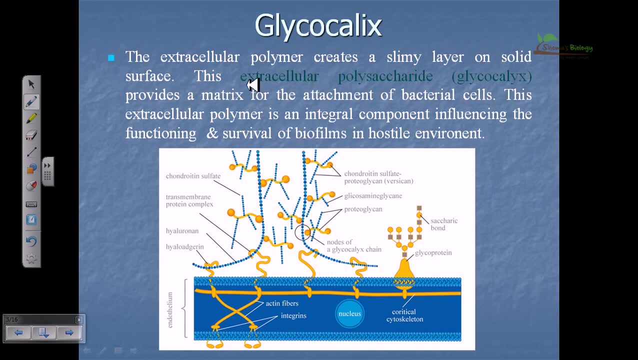 glycocalyx layer is a very, very important layer, because this is giving all the protection to this mats. now, if we look at, uh, the structure of glycocalyx layer, uh, this is simply the extra extracellular polysaccharide layer. okay, so this polysaccharide uh can? 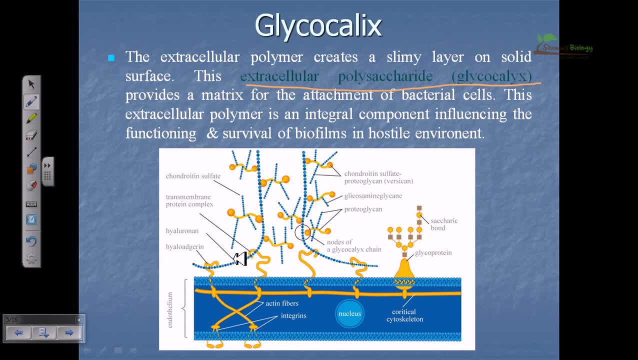 have a protein link to it. so it could be proteoglycan. it could be glycoprotein sometimes and you can find different saccharide balls you can see here. this is a glycoprotein structure. this is the proteoglycan structure here. so normally, normally, what kind of uh structures? 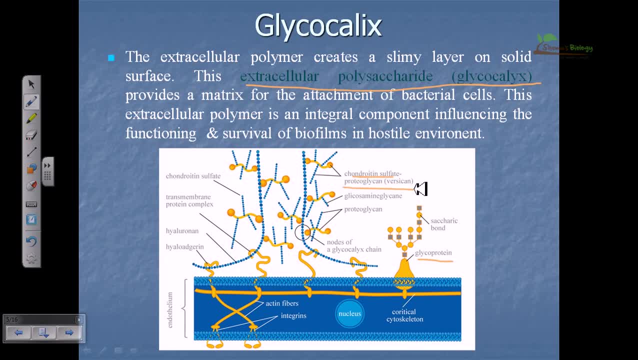 are present here: chondroitin sulfate, uh proteoglycan can be found or heparin sulfate proteoglycan can be found. okay, so chondroitin is a very, very important part. as you can see, chondroitin is a very, very important part, and especially chondroitin sulfate. okay, 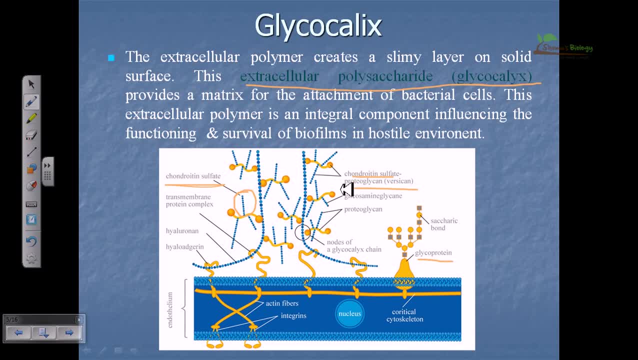 and uh, and also the heparin sulfate is also important. so they take up all those heparin and chondroitin and convert them into chondroitin sulfate or heparin sulfate to make these structures together. so you can find a very, very basic alignment of this glycocalyx layer. 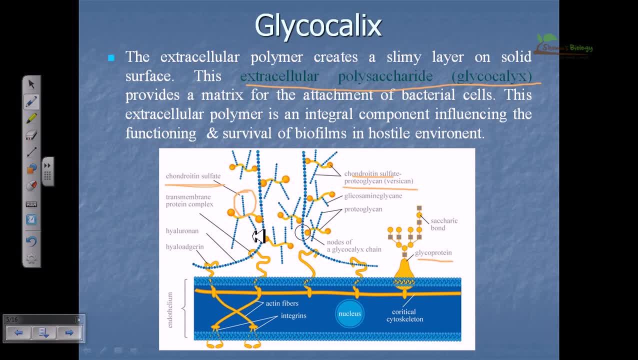 is that, uh, or hyaluronidase, also present in the hyaluron, or all these things? okay, now, here you can find, these are the proteins, and this blue colored thing is the carbohydrate structure. now the proteins are added from one carbohydrate to another, then then other carbohydrates are linked with each other. so what they are doing, they are producing. 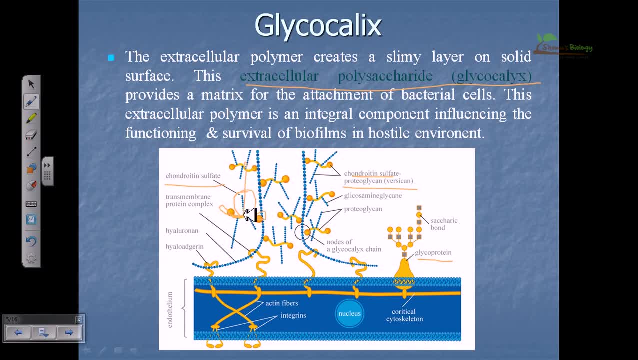 this one structure and this structure will hold on to many carbohydrate chain. so what they are making? they are making a mesh of network, right, a network of this glyco network, of this polysaccharide layers, and it will help them to tightly hold on to the structure of the bacterial cell layer. okay, so it. 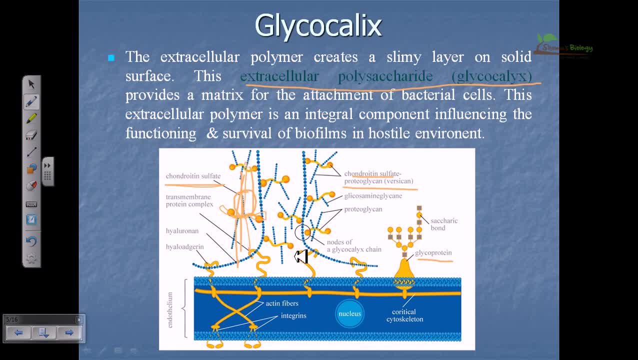 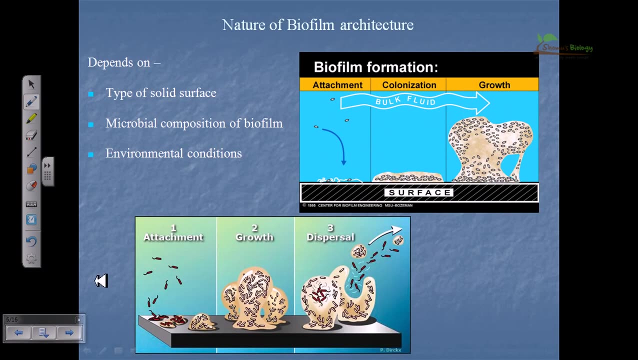 will provide a matrix for the attachment of bacterial cell. okay, so this extracellular polymer is a very, very important component influencing the function of survival of biofilm in the whole hostile environment. that's the basic thing. that's the very, very important thing. the hostile environment, uh, can can have the higher temperature or higher pressure and all these things, but 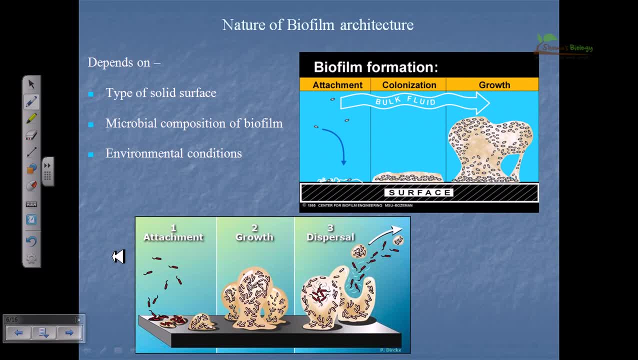 this glycocalyx layer is very, very strong because it is made up with small subunits of monosaccharide, of sugar. okay, now the nature of biofilm architecture: if we look at here, first is the attachment, then colonization, growth and then dispersal, and all these things are very important. 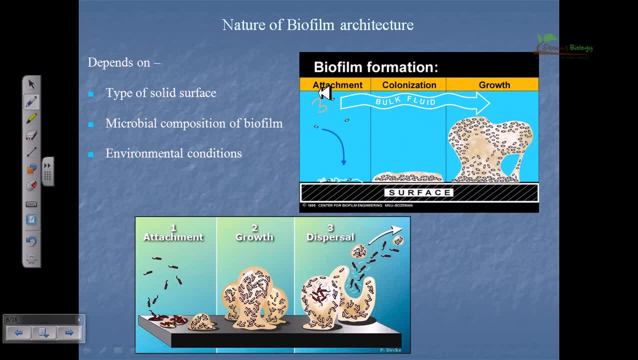 things they must have. the supply of this is the another third most important fact about the biofilm is that they must have the, this continuous supply of bulk fluid. so the fluid flow is also important, otherwise they cannot leave because they cannot move from their own space. so movement is a freeze. so the only way to get all this nutrient is the movement of fluid. so 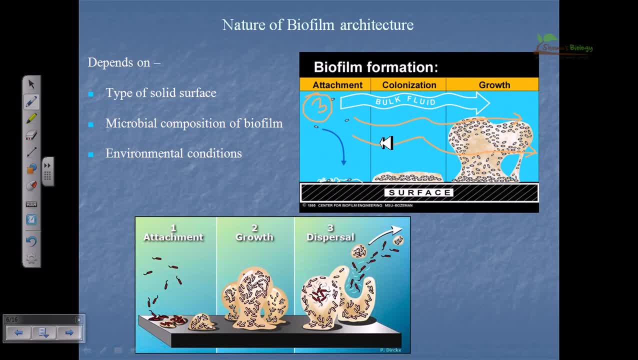 if the movement of fluid is going on, you can find this: biofilms. so, most of the part, when you can find a huge mass of biofilms, in those case you can see that there must be the movement of water movement, movement of water containing nutrients for the bacterial cell. that's a very, very important. 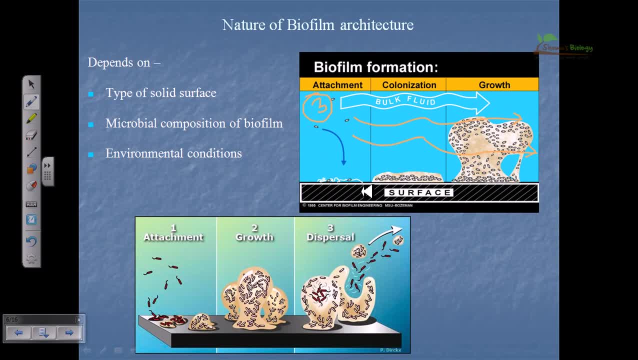 part. so the first important thing is the solid surface, second important thing is the glycocalyx layer and the third important thing is the continuous fluid of continuous movement of fluid containing the nutrient source for the bacterias. now, the nature of biofilm generally depends on this. 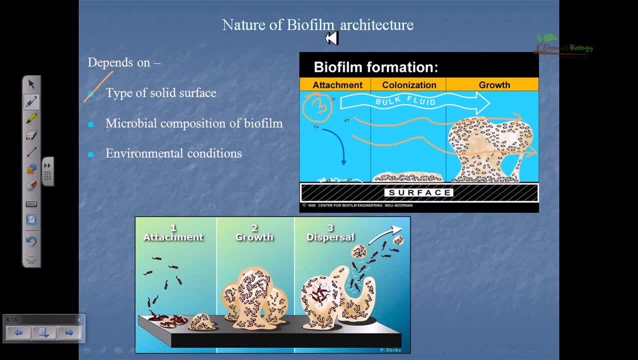 three things: the type of solid surface- uh, these are the nature. so what kind of biofilm we are dealing with can be varied depending upon the three situations. first thing is the type of solid surface. what type of surface these bacteria are actually colonizing, whether this surface can. 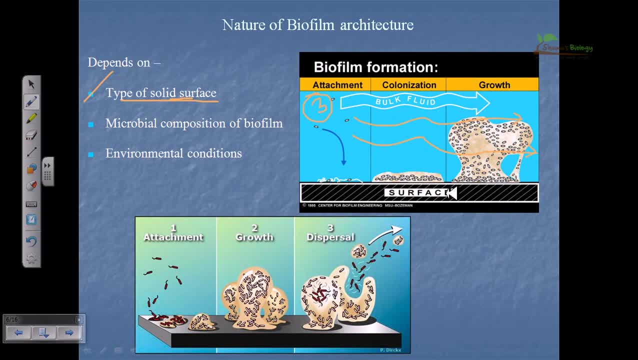 be degradable or it is undegradable. it is very strong or weak, it's soft or hard and whatever it is, it is a first fact. second fact is the microbial composition. if we vary the composition of a biofilm depending upon the variation of the microbe, 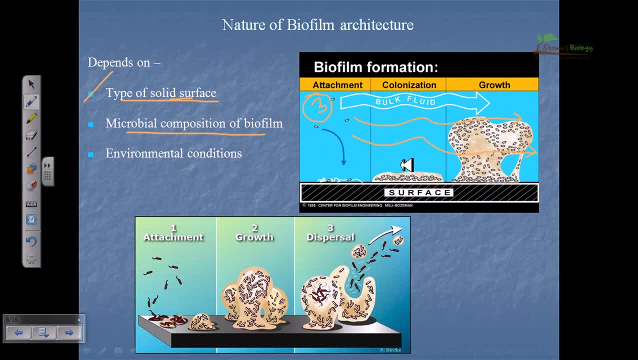 if the microbe THATS in under the body, mass travels between the cial muscle tissue and pedestrian tissue. stories are anib Avengers for womenavait unknown where there is a product specific for one to many people in the form of theécole. no, we are estimating the responsibility of 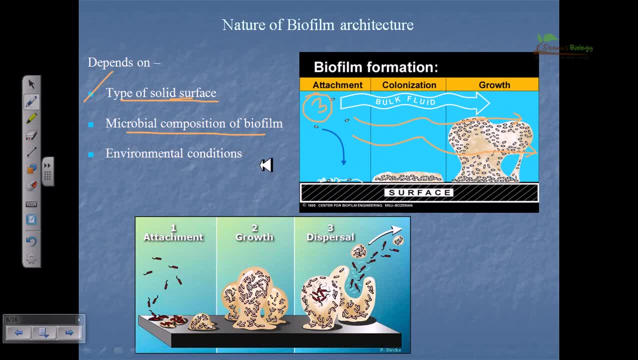 topography. so even if the palms are not, becomes autologous, but do not contract that the appearance of the central and the Süd. the same is true when we develop this type of кам trailer. remove them on the on the mechanical uh use of mechanical uh forces. so it's very, very difficult. 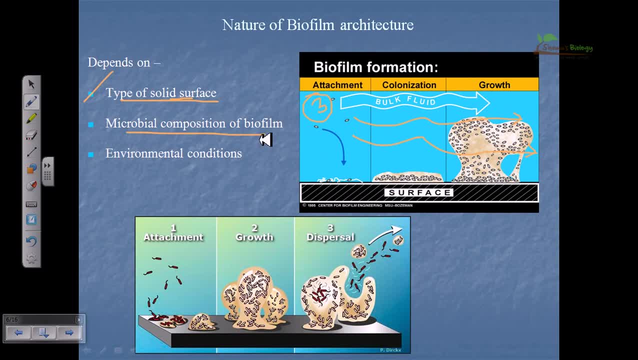 right? so how much tightly they are attaching on those spaces? this is very, very dangerous. the third part is the environmental condition. that's the most important part, because the environmental condition will dictate what type of thing you are doing, because whatever you are doing, wherever you are staying, it depends on the environment, right? so these three things dictate. 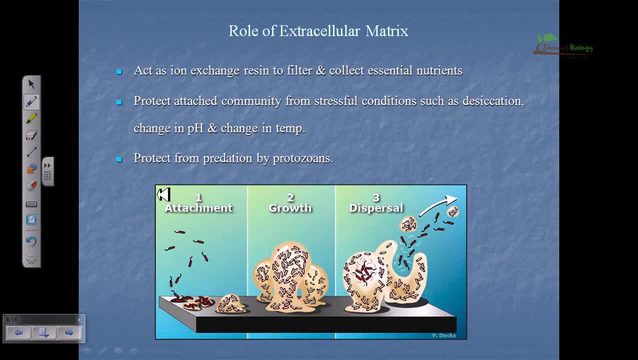 the architecture and the nature of biofilm that we are dealing with, and we have talked about the glycocalyx a little bit, uh, but now let's talk about the role of this extra extra cellular matrix right, which is also made up with glycocalyx layer. now it act as an ion exchange resin. that's very important.